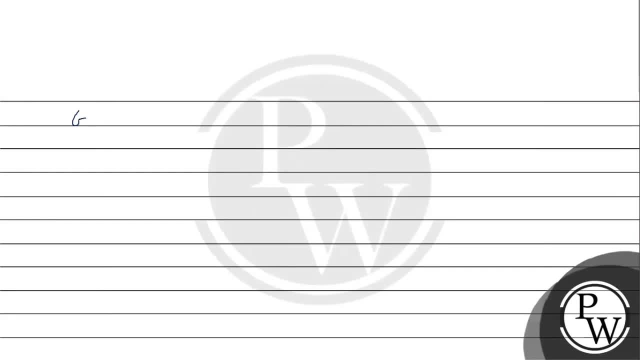 of our function Given. what is the function given to us? f of x is equal to mod 3x minus x, square plus 2 minus x. And what is the interval given? Closed interval minus 1 comma 2.. x belongs to closed interval minus 1 comma 2.. So, first of all, we will tackle this mode. 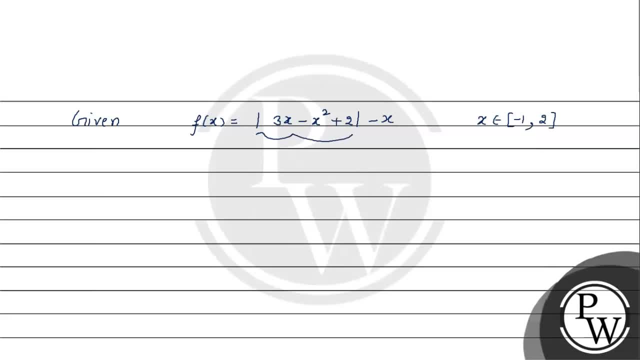 For this mode. we will solve it. Which values of x will come? See, you can solve it roughly: x square minus 3x plus sorry, minus 2 is equal to 0.. I took minus out. you keep it. 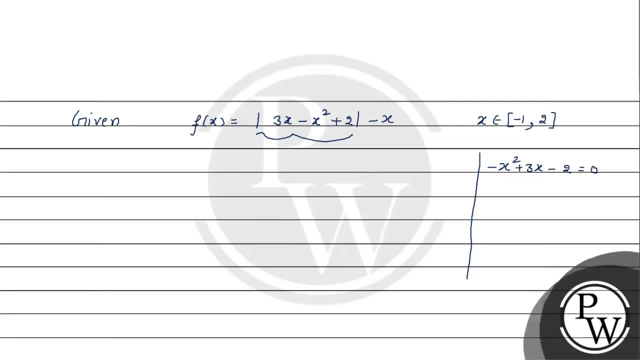 minus minus x square, or keep it here, only Plus 3x, and this plus 2 is equal to 0.. So it will be minus 2.. This is given to us From here. I will solve for x, So I will get. 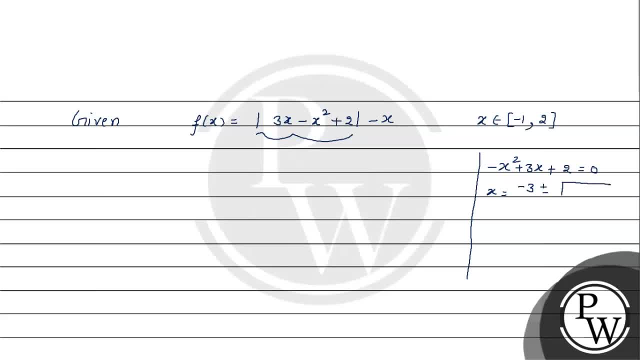 minus b plus minus square root of b square, that is 9 minus 4, a will be minus 1 and c will be 2.. Divided by 2a, a is minus 1.. So it will be minus 3 plus minus square root. 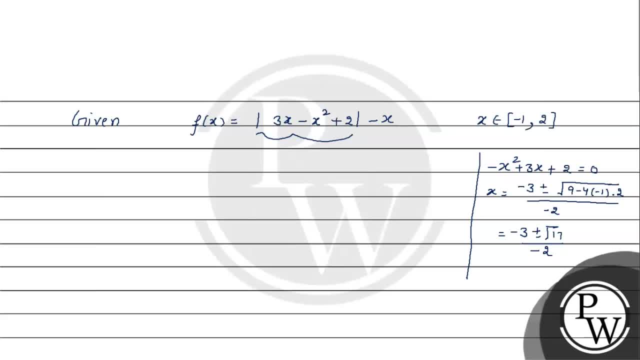 17 by minus 2.. So when you take minus from above, then it will be minus 3 plus minus square root, 17 by 2.. So from here we got two values of x. We got one value of x, 3 plus. 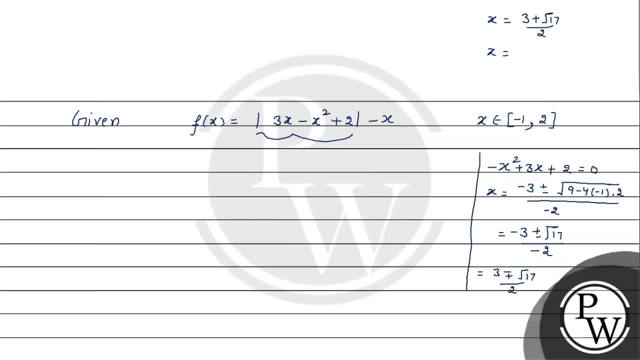 square root 17 by 2.. And the second value we got, x, is equal to 3 minus square root 17 by 2.. When you solve this value, see, the square root is 17,. that is our 4.123.. So 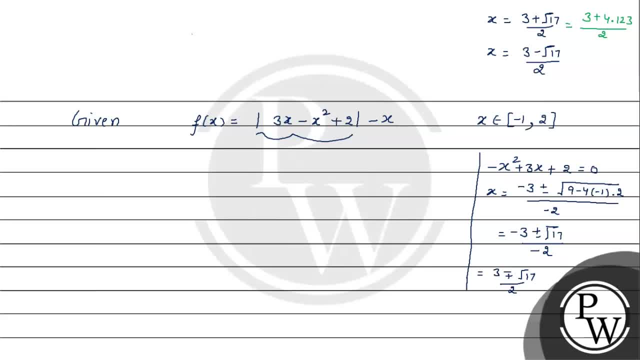 if we divide it by 2, then our interval, which is our interval, will go out from minus 1 to 2.. So we will not take this value, we will reject it. This value is left. this will come, if you solve it, then minus 0.56.. So it will lie in between this. So we will take. 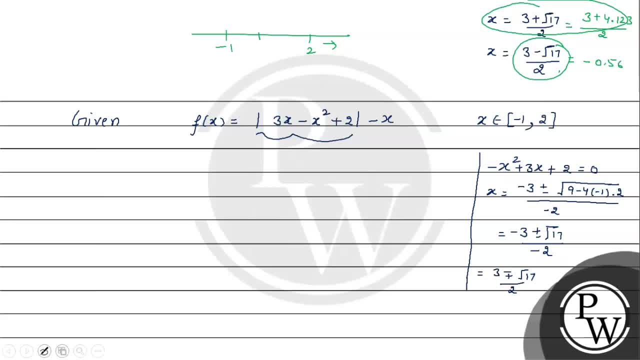 this value of x, That is our function, will be split on this. So our interval, which was minus 1 to 2, where the function was split in between, that is 3.. So we will take this minus square root, 17 by 2.. So what is our fx function now? f of x is equal to when it. 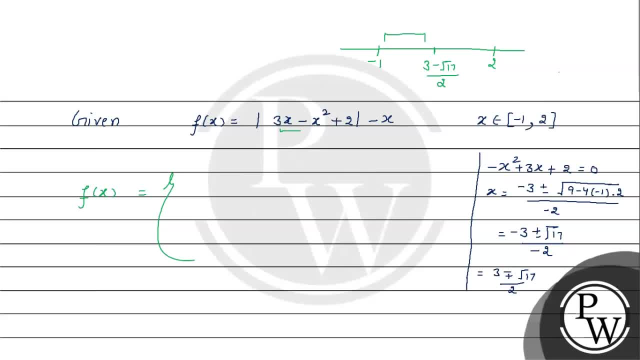 will be in this interval, then how will this value come? It will be negative. So if you put minus outside, it will become 3x minus x square plus 2.. And this was minus x outside When x belongs to closed interval minus 1, to where 3 minus square root 17 by 2.. So 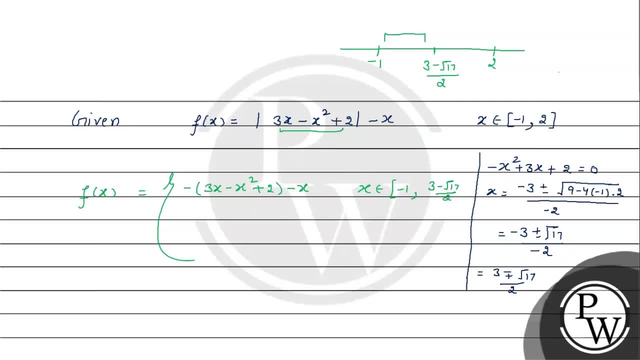 it will be 3 minus square root, 17 by 2.. And this value will be 3x. It will be positive here for this interval And minus x was there at the back, So it will give x belongs to here. I will include it: 3 minus square root, 17 by 2 comma 2.. Now our f of x has become: 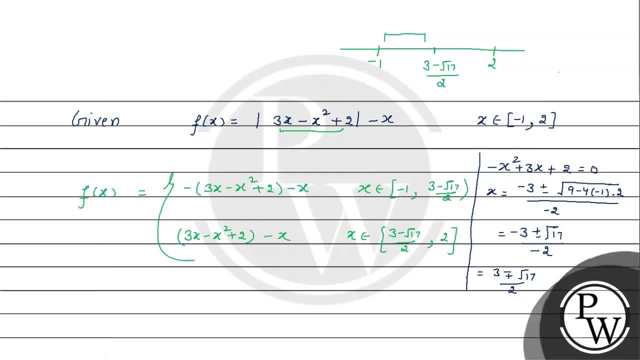 a split function. If I write it by solving it, then it will become see x square minus 4x minus 2.. And this function will become. what will it become? It is in equality, only It will become minus x square plus 2x plus 2.. Now we will find out: f dash x, f dash x. 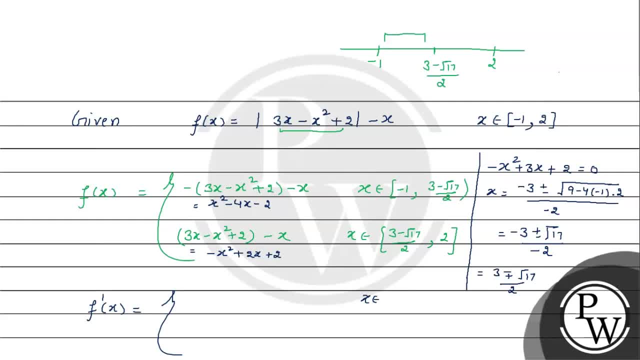 if for this interval of the above function, when x belongs to closed interval minus 1 to here I have taken semi open 3 by, by the way, a semi value will come from both. If you include it, then what will be my derivative? here 2x minus 4.. And here the derivative. 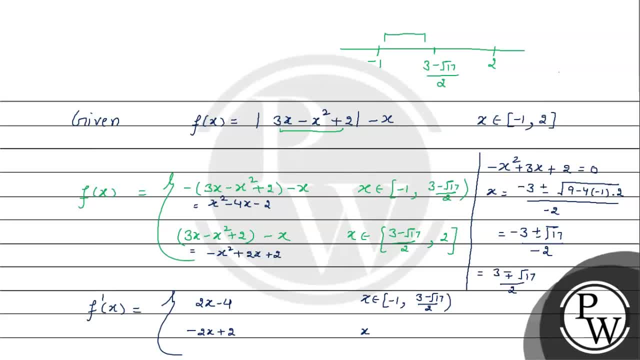 will be minus 2x, plus 2 when x belongs to closed interval 3 minus square root 17 by 2 comma 2.. Now we have to find out the stationary point. For the stationary point, once I will keep this f dash x as 0.. Once we keep this f dash equal to 0, then only it will come out. 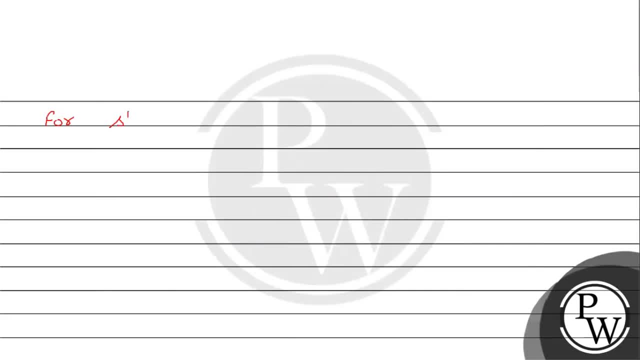 4. Stationary point, when x belongs to closed interval minus 1, and here I have taken semi open 3 minus square root, 17 by 2.. For this interval, what was our f dash? x, 2x minus 4.. 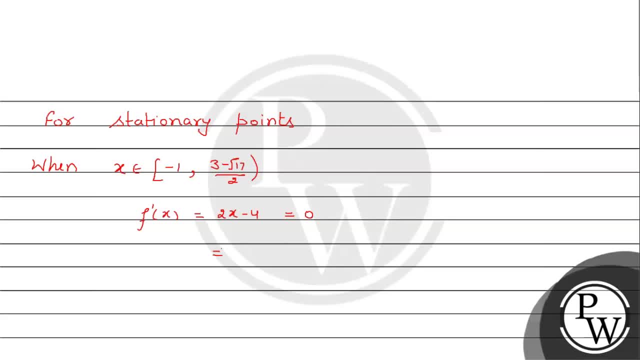 I took this equal to 0. This implies: what did we get from here? 2.. So what did we get? We got the critical point, We got its stationary point. Now we will check the value of the function on these three points. Which are the three points? Two are the points of our interval. 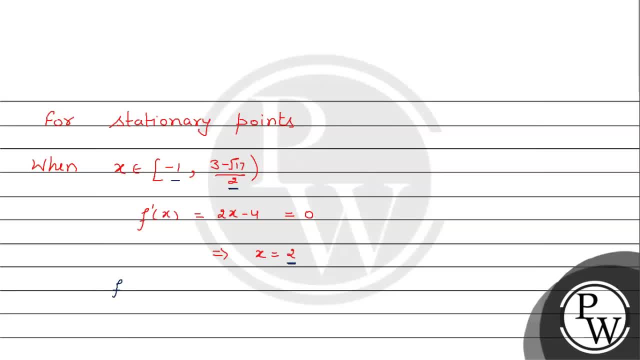 ending point, and one is this point: So if you check the value of the function on f of minus 1,, then what will we get? This value will be given on f of minus 1, 3.. And if you check on f of 2,, then this value will be given to us 2. And this value will be given to us. 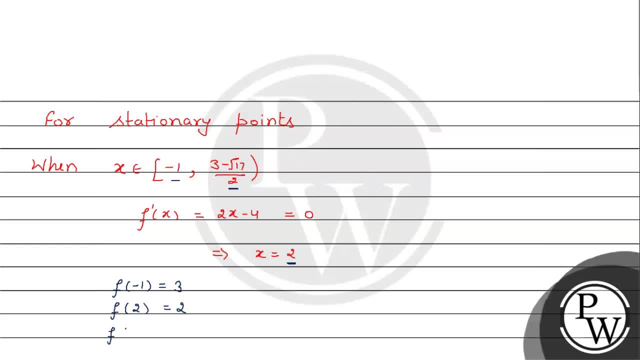 2.. And when you check the value of the function on f of 3 minus square root 17 by 2, then this value will be given to us: square root 17 minus 3 by 2.. Because f of x, you have to take this. 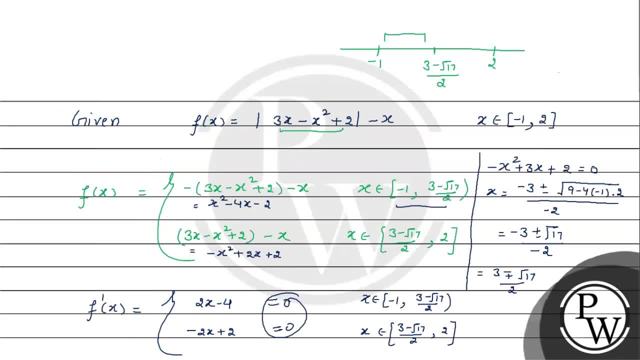 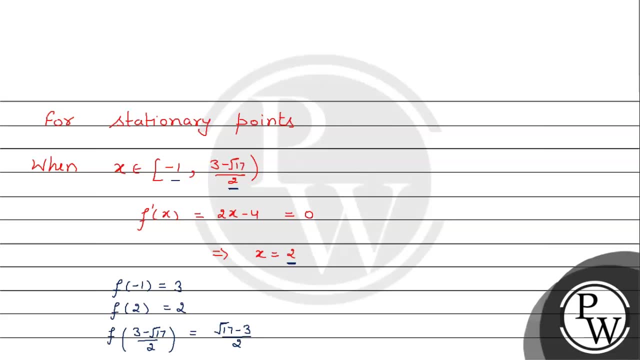 one. What interval are we talking about? We are talking about this interval. So f of x, you will take this one. We will check for this interval. When you put it on this, then it will give us these values. One more thing: what is x here? It is 2.. And we have f dash. 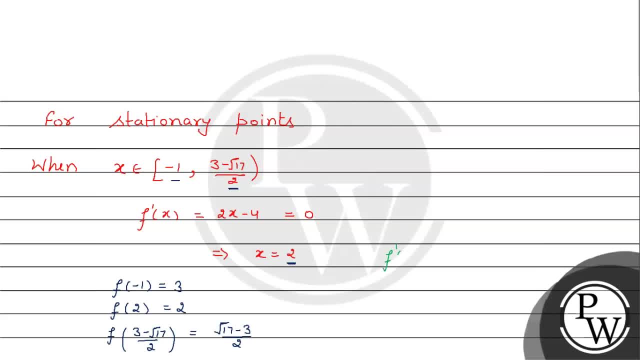 x. What is f dash x? It will be f dash x. If I take two commas, then it will be x minus 2.. This implies that our f dash x in this interval, in this interval, is always decreasing, Decreasing. 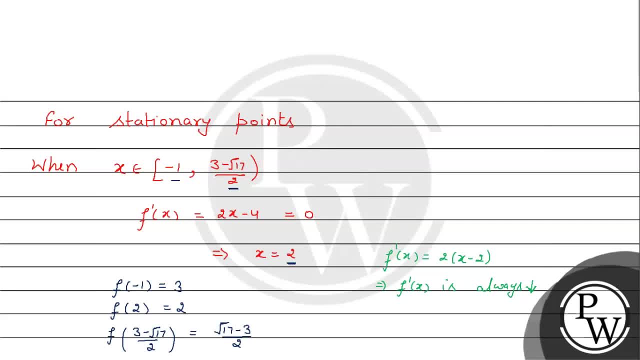 Decreasing, Decreasing. So here we will get the minimum value. What is the minimum value? It has been given at this point, And this is our minimum value, Because I had just told you that square root 17 will be 4.123 minus 3.. This will be one point something, And if we divide it by 2,. 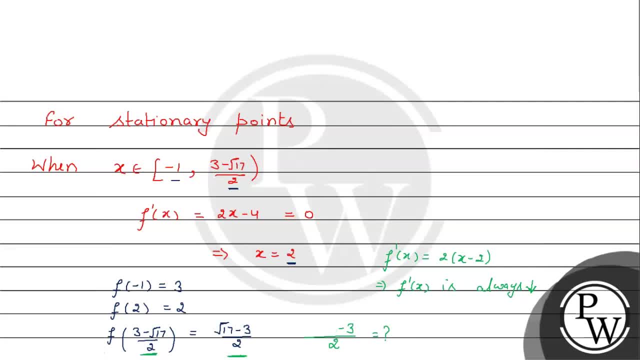 then it will go smaller. Just this is the calculation part. The value you have to keep is this: square root 17 minus 3 by 2.. Now we will remove the 2nd stationary point when x belongs to minus- sorry, 3 minus square root 17 by 2. 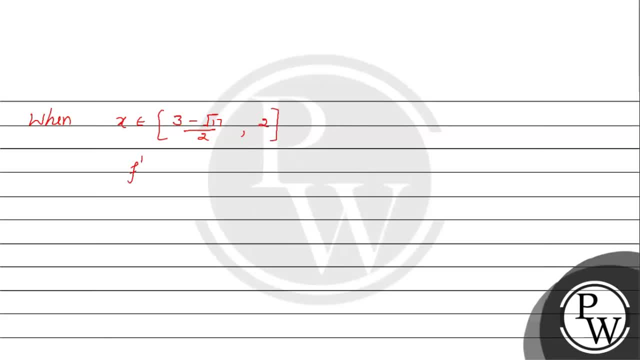 till 2. in that case, f dash x is minus 2x plus 2. we will keep it as 0 to get the stationary point. this implies from here we will get x, we will get 1. now, what are the points we have when we will find the value of the function? 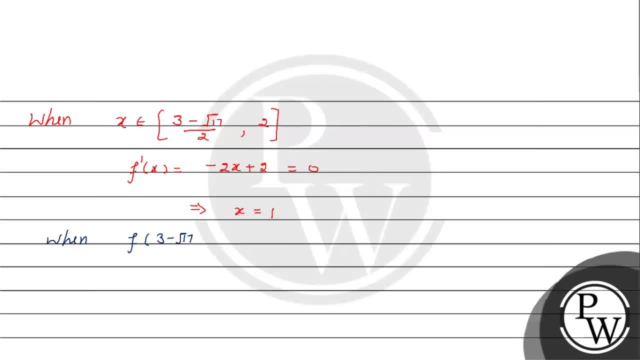 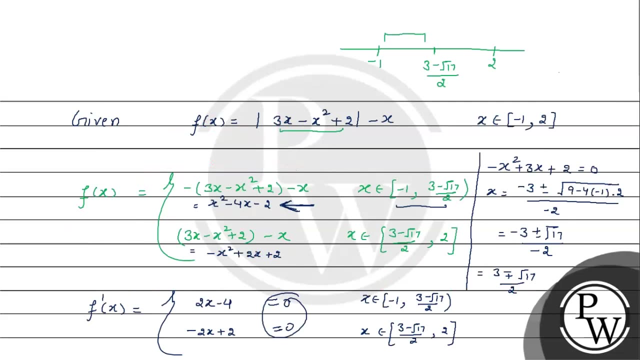 3 minus square root 17 by 2. on this, our value will be same. as we have found square root 17 minus 3 by 2, we will find out the value on f of 2. f of 2 will give this value. see, you will keep x as 2. 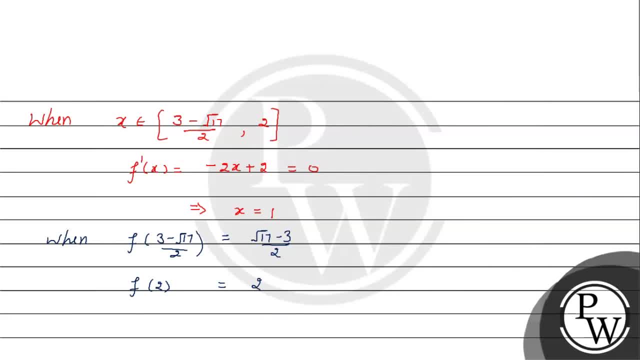 so this 2 value will be given and on f of 1, this value will be given. so from here, if we see, the maximum value we got is 3, absolute maximum value. and absolute minimum value we got is square root 17 minus 3 by 2. 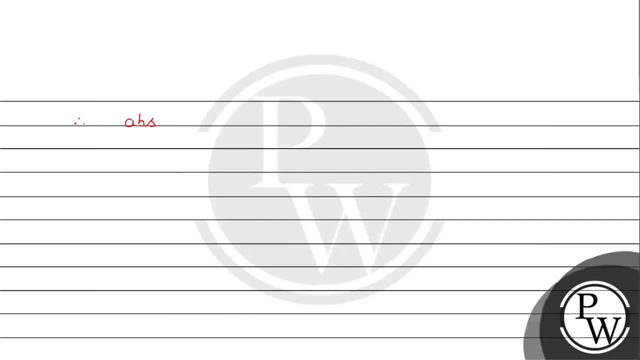 therefore, absolute maximum value- we got absolute maximum value is 3 and absolute minimum value is 3 and absolute maximum value is 3 and the absolute minimum value is square root: 17 minus 3 by 2, we got the sum. what will be the sum? 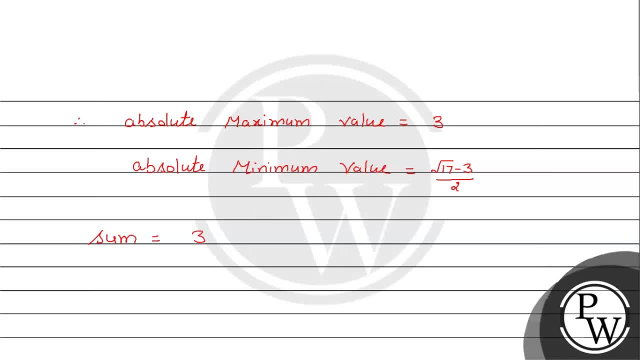 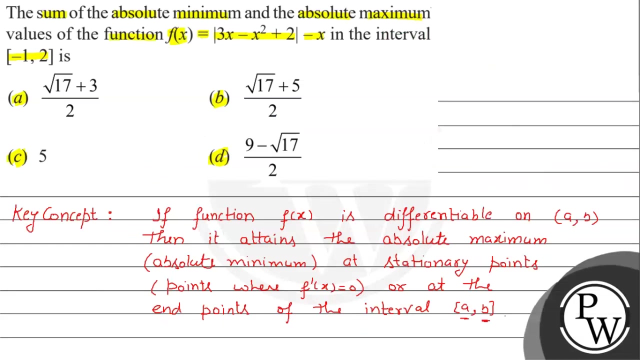 sum is equal to 3 plus square root 17 minus 3 by 2. you add it and solve it. we will get square root 17 plus 3 by 2. This implies option A is correct. Option A is correct and all other options are incorrect. Hope you understood it well. Best of luck.